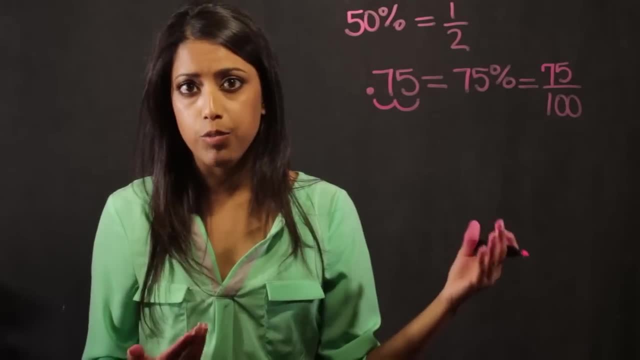 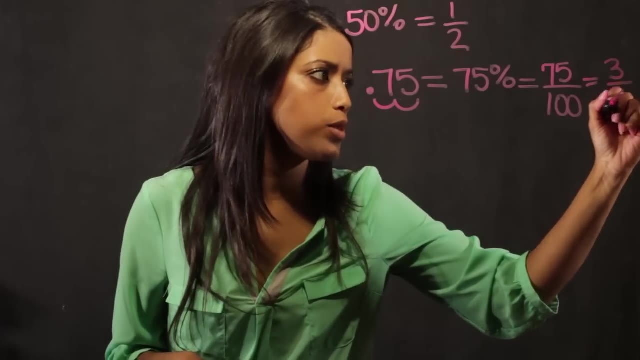 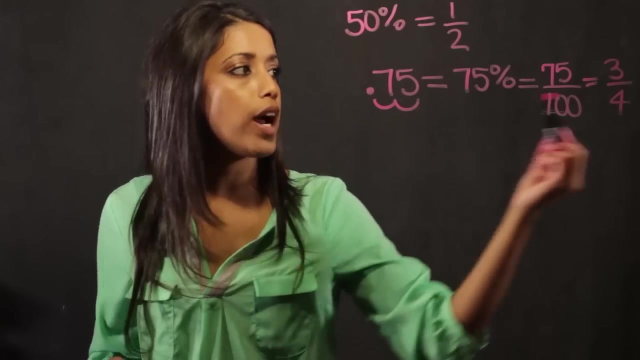 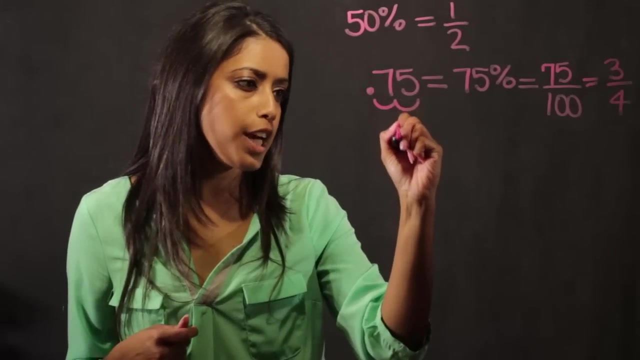 what numbers do they have in common? 75 is divisible by 25.. It goes into 75 three times. 25 goes into 100 four times. So the fraction that represents 75% and also .75 is three-fourths. Let's just do a few more examples, If I take. let's start with a fraction, Let's take one-fifth. 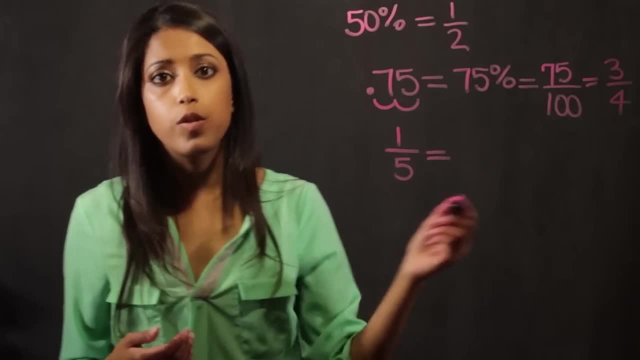 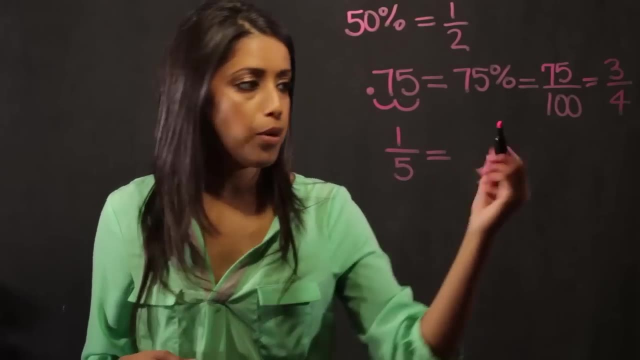 And let's say that I want to convert that to a decimal point. The way that we convert to a decimal point is by taking the top number and dividing it by the bottom number. So I'm going to take one and I'm going to divide it by five. Five doesn't go into one, so we 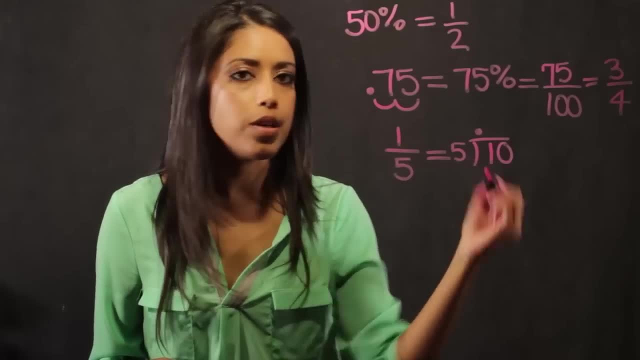 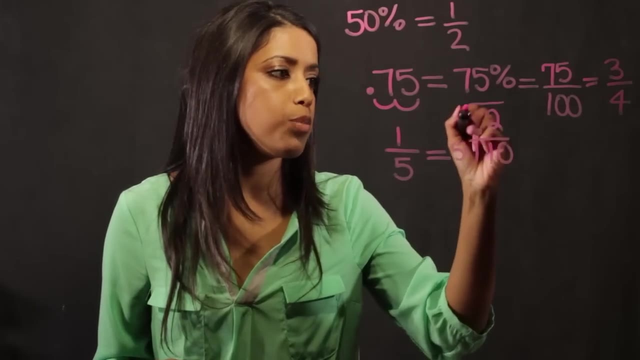 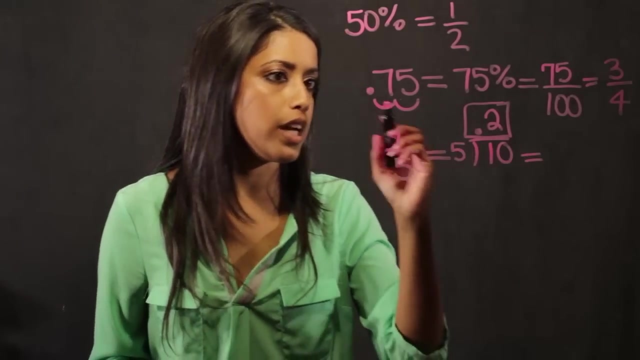 have to add a decimal point here, And that allows us to put a zero there. Five goes into ten two times, So our decimal point for one-fifth is .2.. Now it's time to add a decimal point. It's time to convert this to a percentage. The way we convert from a decimal to a percentage. 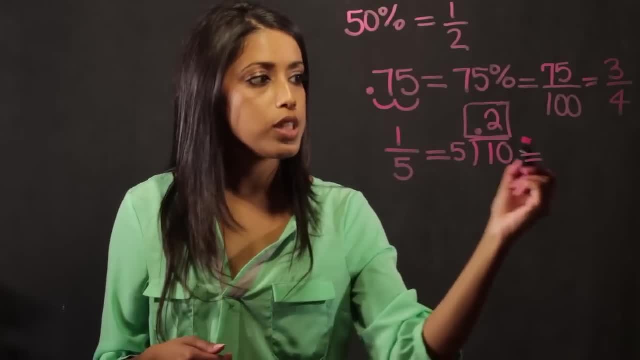 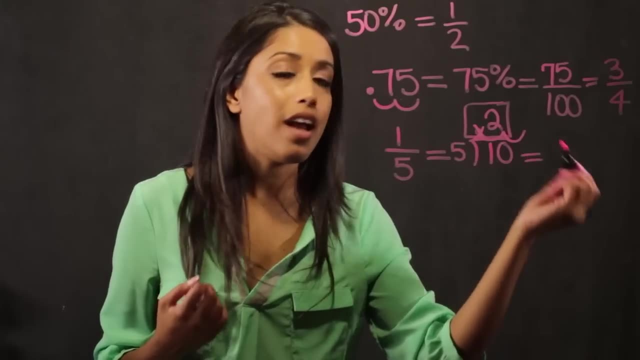 is the same way we did up here, where we moved that decimal place two times. So I'm going to take the decimal and I'm going to move it one, two, I'm going to drop my decimal and add the percent sign And fill in any spots with a zero. So this is going to become: 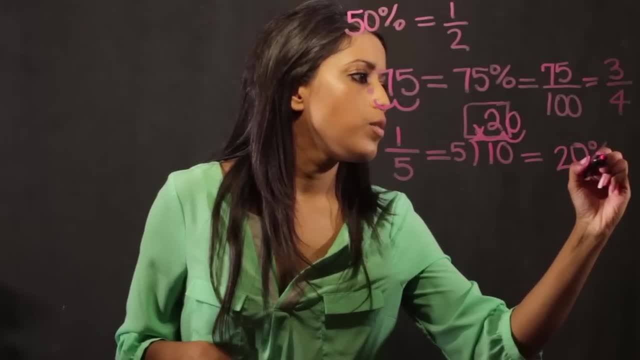 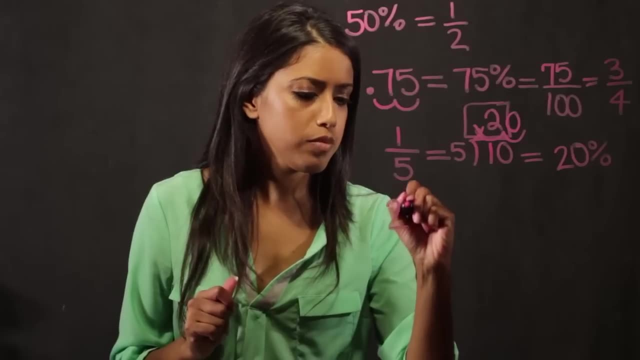 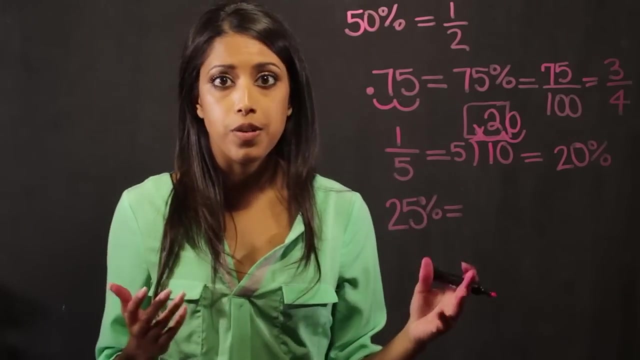 twenty percent. Let's go ahead and do one final example. Let's take twenty percent, Twenty-five percent And let's convert it. So we're beginning with the twenty-five percent And let's say we want to convert that to a fraction, When it's already in percentage. 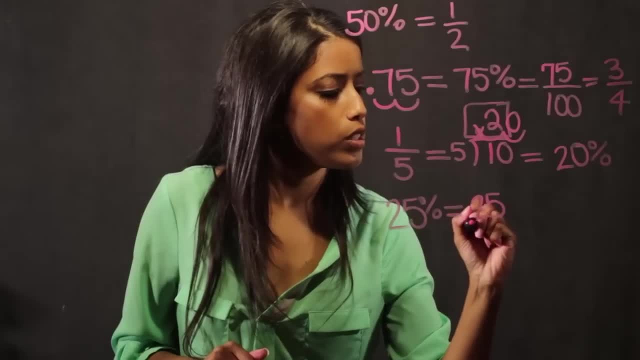 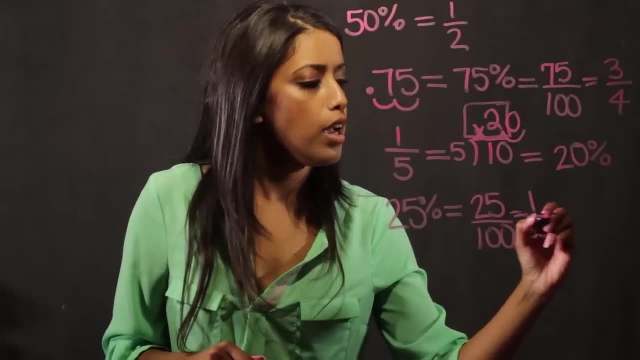 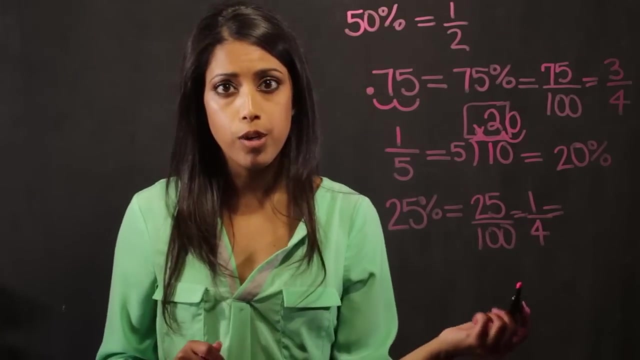 form. we just take it and we put it over a hundred, So this becomes twenty-five over a hundred, And when we reduce, we know that twenty-five goes into itself one time and it goes into a hundred four times. Now what we want to do is put it into a decimal form. 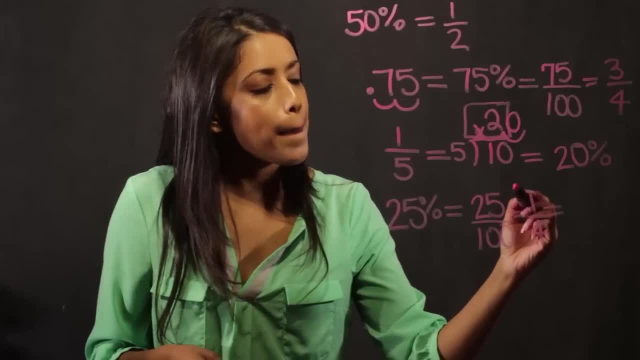 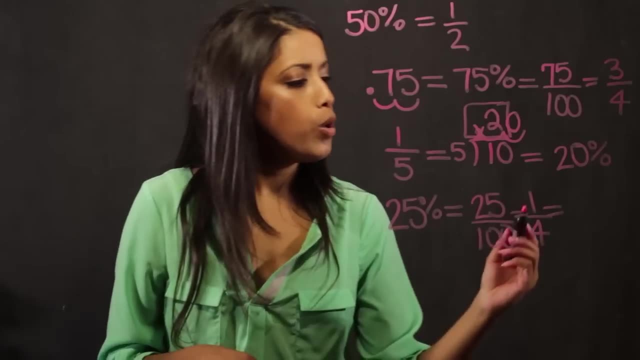 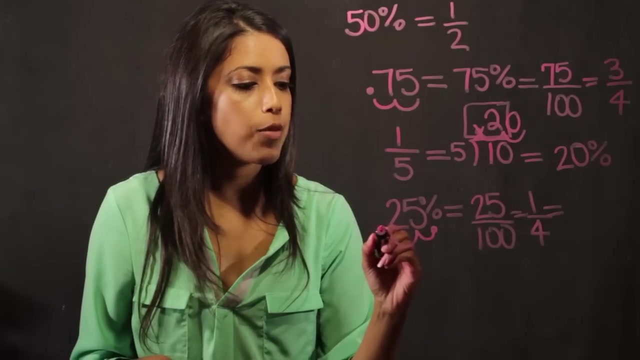 Now there's two ways that we can do this. We can do it where we divide the top number by the bottom number, and we can also use the percentage and just move the decimal point. If we use the percentage, basically what we do is we take the decimal and we move it to the left, One, two And we add it. So we know.